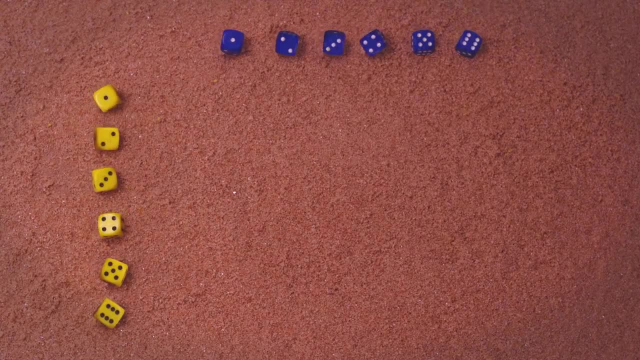 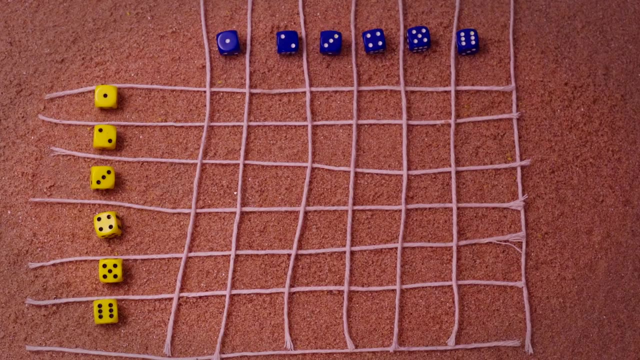 Now we can see why the first glance was wrong. Even though player one has four winning numbers and player two only has two, the chance of each number being the greatest is not the same. There is only a 1 in 36 chance that 1 will be the highest number. 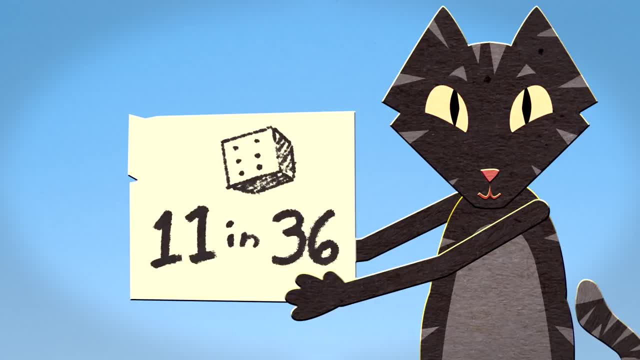 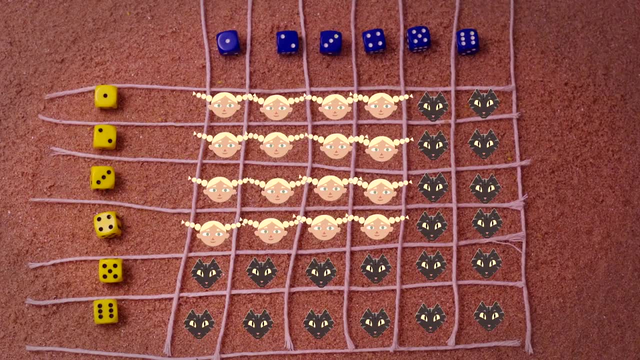 but there's an 11 in 36 chance that 6 will be the highest. So if any of these combinations are rolled, player one will win. But if any of these combinations are rolled, player two will win Out of the 36 possible combinations. 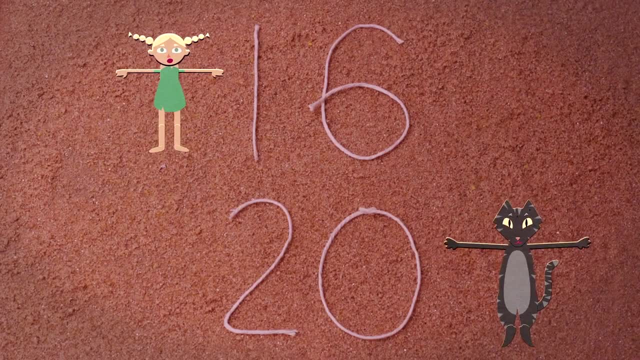 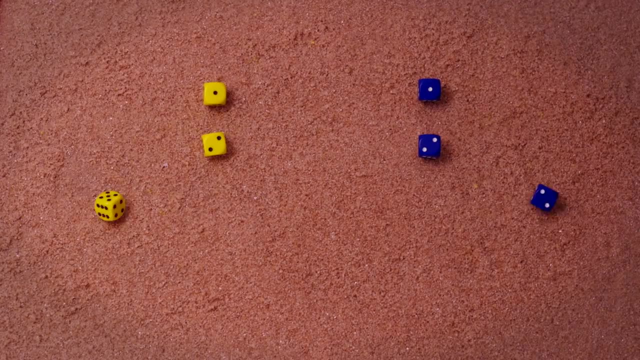 16 give the victory to player one and 20 give player two the win. You could think about it this way too. The only way player one can win is if both dice show a 1,, 2,, 3, or 4.. 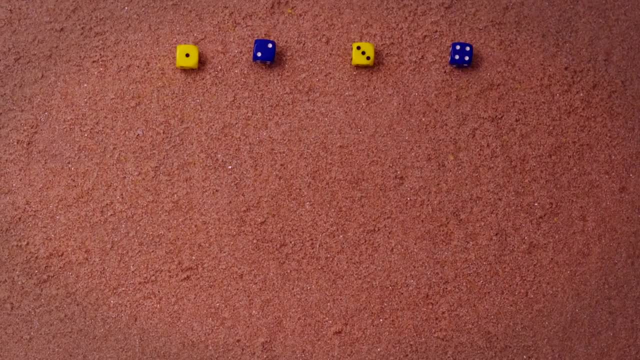 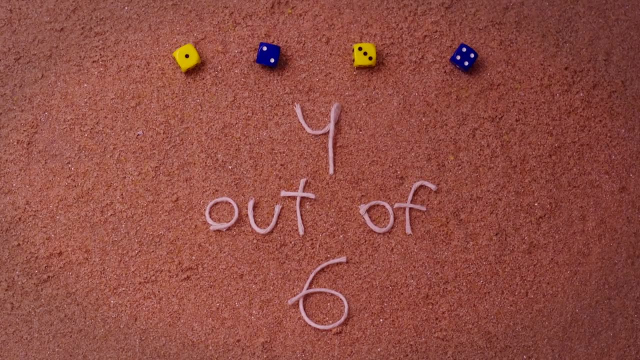 A, 5 or 6 would mean a win for player two. The chance of one die showing 1,, 2,, 3, or 4 is 4 out of 6.. The result of each die roll is independent from the other. 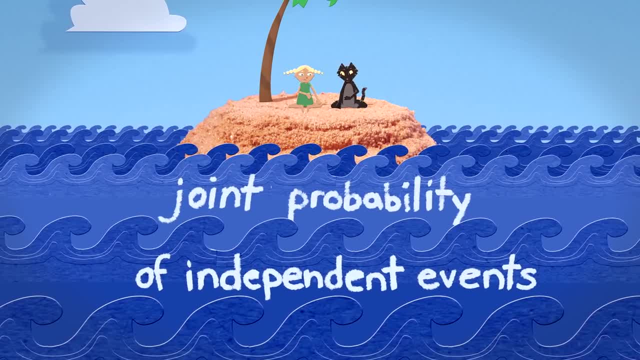 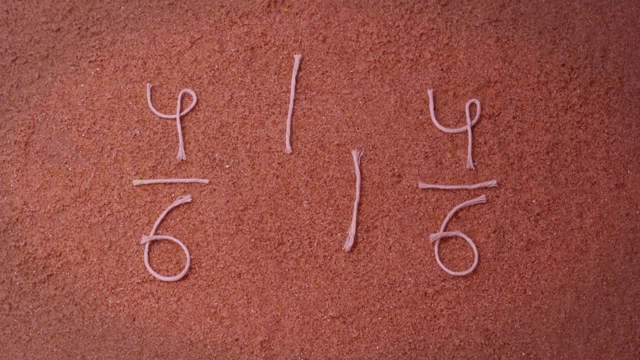 and you can calculate the joint probability of independent events by multiplying their probabilities. So the chance of getting a 1,, 2,, 3, or 4 on both dice is 4 out of 6 times 4 out of 6, or 16 out of 36.. 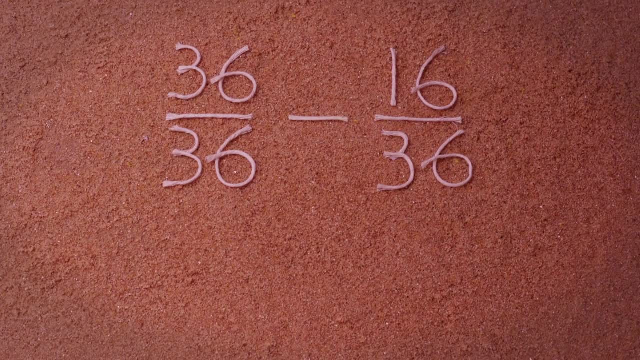 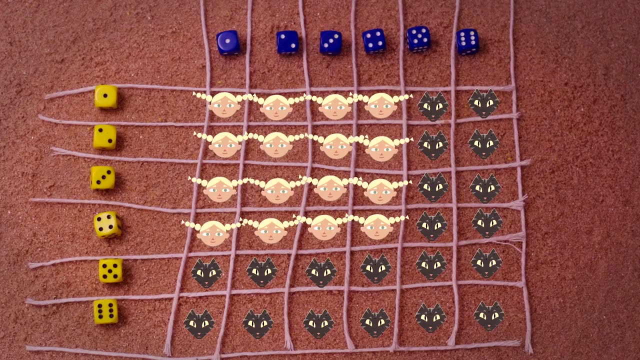 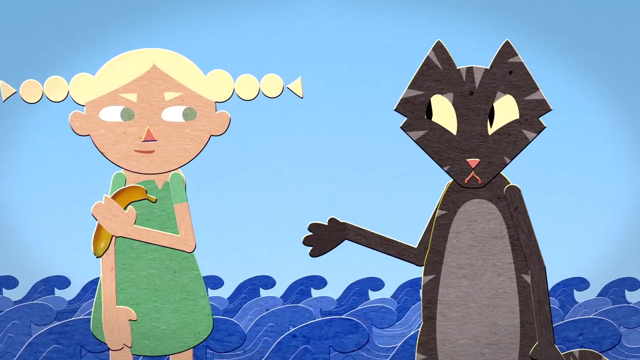 Because someone has to win. the chance of player two winning is 36 out of 36 minus 16 out of 36, or 20 out of 36.. Those are the exact same probabilities we got by making our table, But this doesn't mean that player two will win. 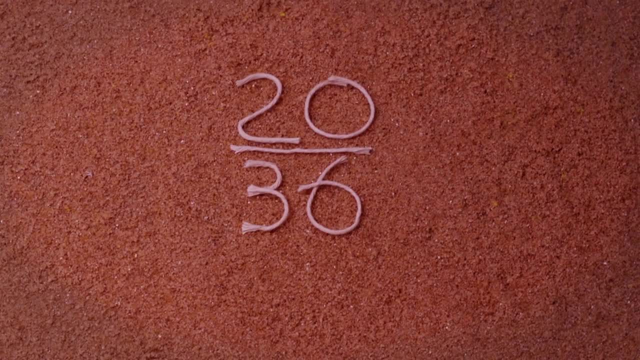 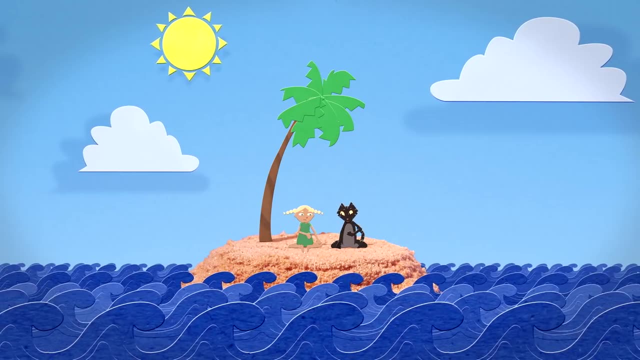 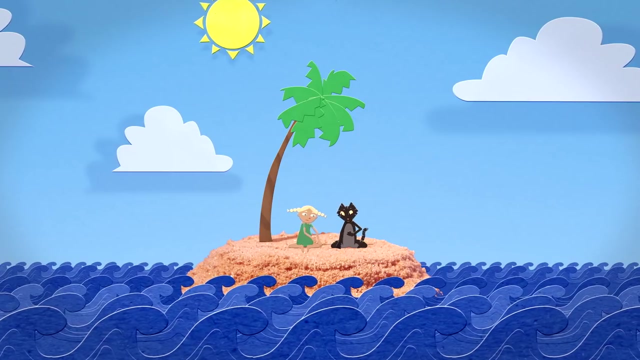 or even that if you played 36 games as player two, you'd win 20 of them. That's why events like dice rolling are called random. Even though you can calculate the theoretical probability of each outcome, you might not get the expected results if you examine just a few events. 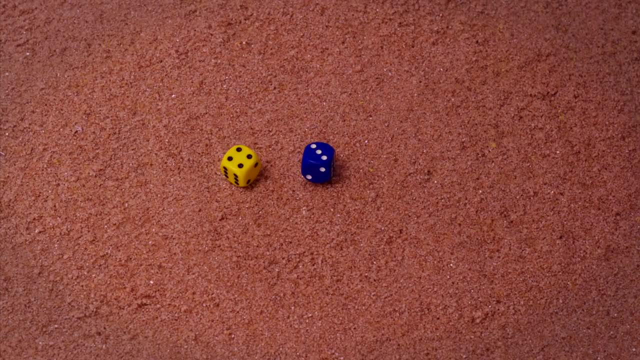 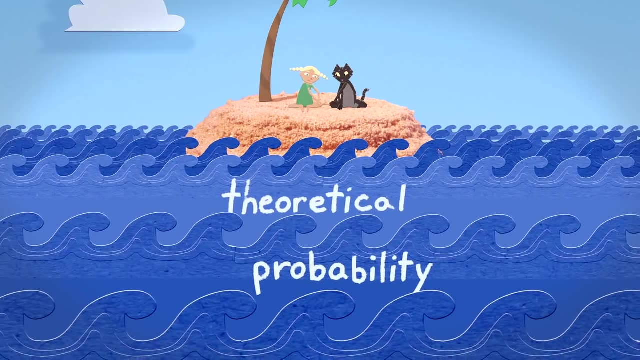 But if you repeat those random events many, many, many times, the frequency of the game will increase. The frequency of a specific outcome, like a player, two win will approach its theoretical probability, that value we got by writing down all the possibilities.